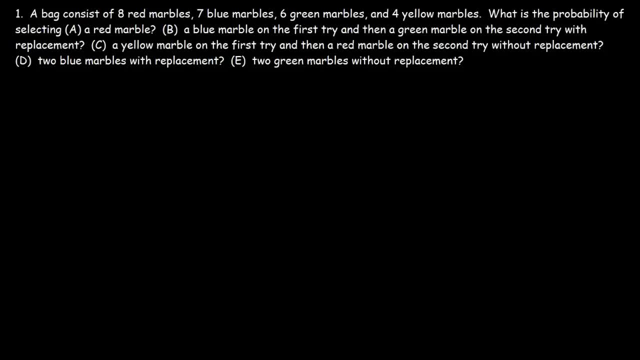 video and go ahead and do so. So let's begin. Let's write out the marbles that we have. So the first color is red, the second color is blue, the third color is green and the fourth color is yellow. So you can clearly see the information. Now we have eight red. 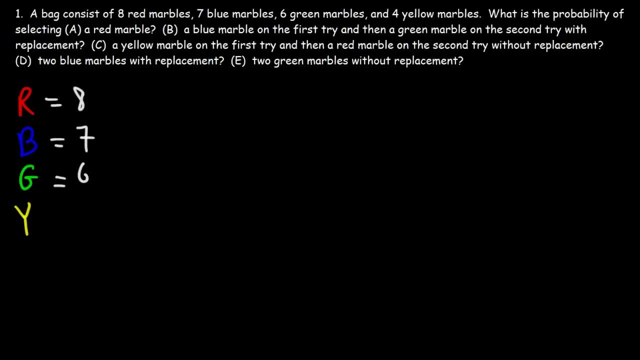 marbles, seven blue marbles, six green marbles and four yellow marbles. Now let's get the total. Six plus four is ten. Eight plus seven is fifteen. Fifteen plus ten is twenty five, So we have a total of twenty five marbles. So what's the probability of selecting a red marble? 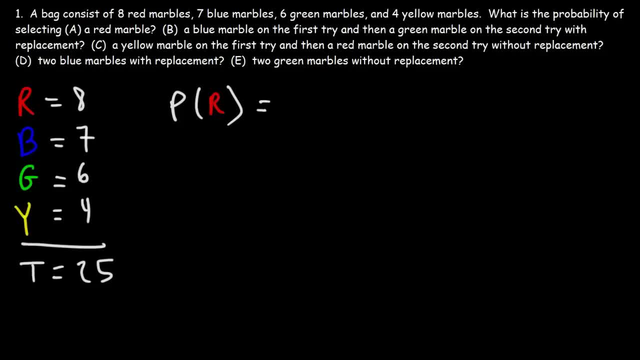 To calculate the probability of an event occurring. it's basically the number of favorable outcomes divided by the total possible outcomes. In this case it has to do with marbles, So it's going to be the eight red marbles that we have divided by the total number of marbles. 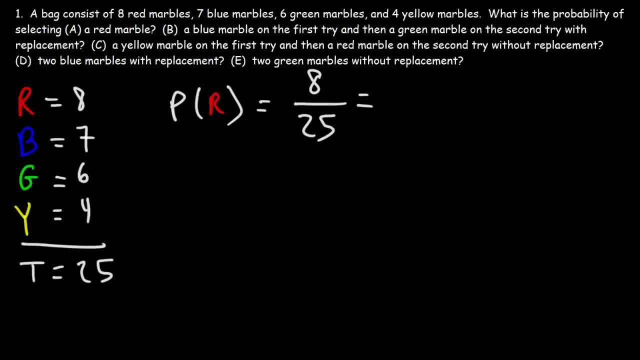 which is twenty five. Eight divided by twenty five is point three, two. So what this means is that there's a thirty two percent chance of selecting a red marble on the first try. Now what about part b? What is the probability of selecting a blue marble on the first try? 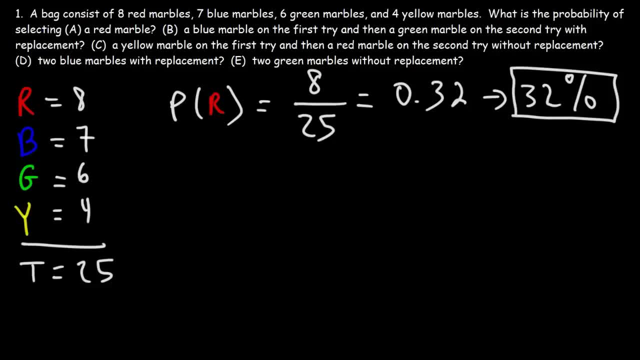 and then a green marble on the second try with replacements. So what is the probability of getting b and then getting g? So let's do this one at a time. The probability of getting a blue marble is going to be the number of blue marbles, which is seven divided by 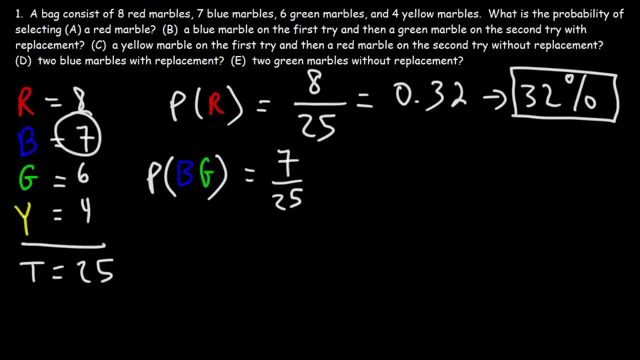 the total number of marbles, which is twenty five. Now, what about the green marble? Well, we need to understand the expression with replacement. So that means that once we select the blue marble on the first try, we're going to put that blue marble back in the bag. So we still have a total of twenty five marbles, And there. 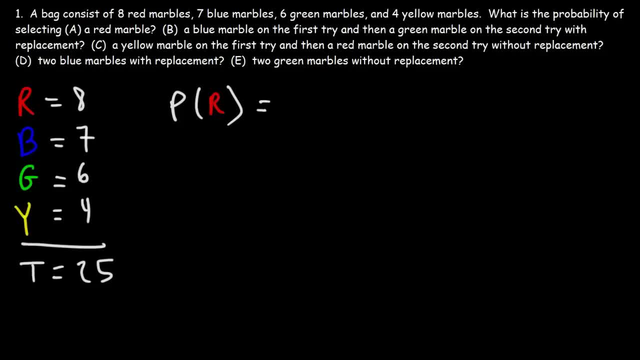 To calculate the probability of an event occurring. it's basically the number of favorable outcomes divided by the total possible outcomes. In this case it has to do with marbles, So it's going to be the eight red marbles that we have divided by the total number of marbles. 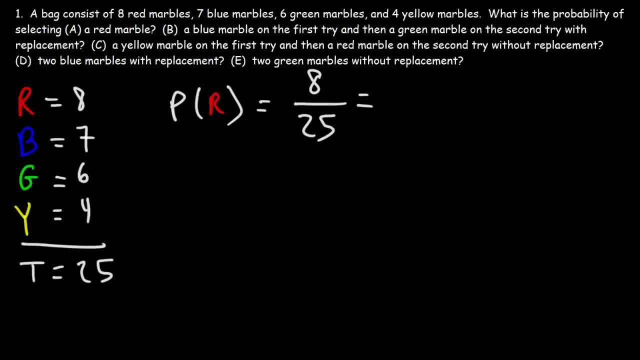 which is twenty five. Eight divided by twenty five is point three, two. So what this means is that there's a thirty two percent chance of selecting a red marble on the first try. Now what about part b? What is the probability of selecting a blue marble on the first try? 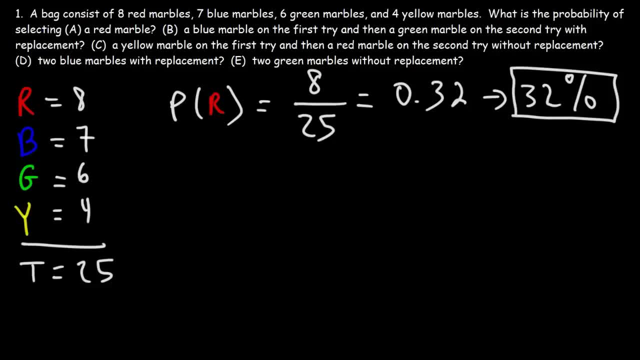 and then a green marble on the second try with replacements. So what is the probability of getting b and then getting g? So let's do this one at a time. The probability of getting a blue marble is going to be the number of blue marbles, which is seven divided by 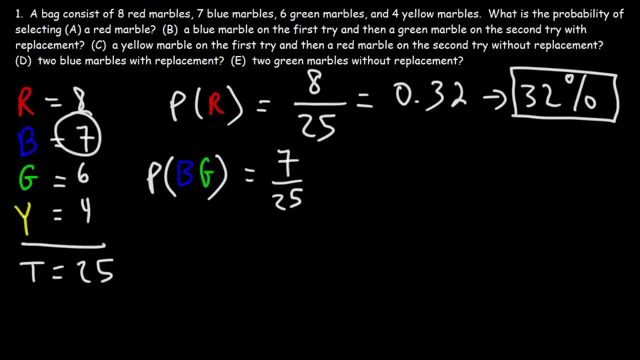 the total number of marbles, which is twenty five. Now, what about the green marble? Well, we need to understand the expression with replacement. So that means that once we select the blue marble on the first try, we're going to put that blue marble back in the bag. So we still have a total of twenty five marbles, And there. 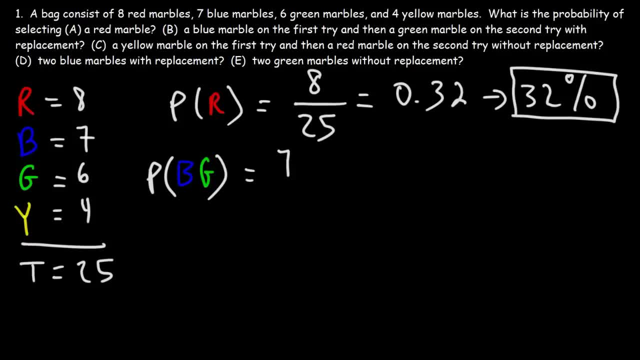 are six green marbles. So the probability of getting a green marble will be six out of twenty five. So now let's do the math. Seven times six is forty two. Twenty five times twenty five is six hundred and twenty five. Now, forty two divided by six twenty five, that's point zero. six seven. 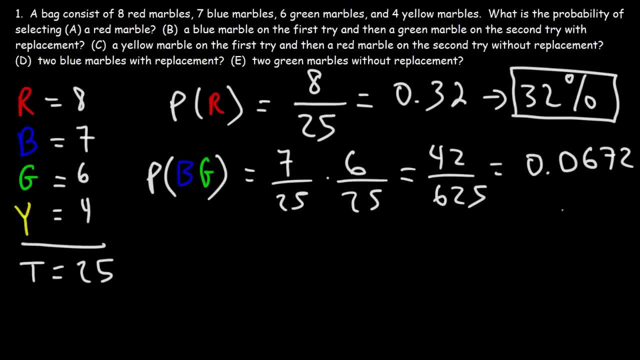 two. So if we multiply that by a hundred, that corresponds to a six point seven, two percent chance of getting a blue marble on the first try and then a green marble on the second try. Now let's move on to part c. What is the probability of selecting a yellow marble on the first? 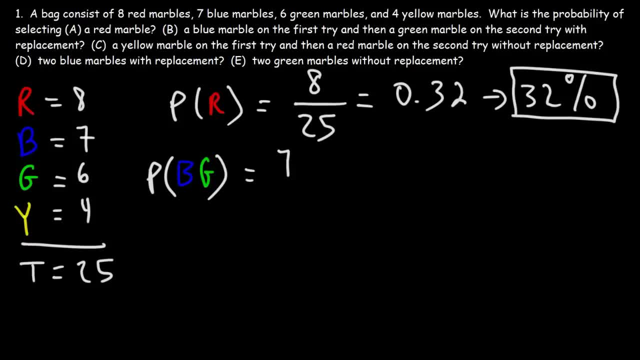 are six green marbles. So the probability of getting a green marble will be six out of twenty five. So now let's do the math. Seven times six is forty two. Twenty five times twenty five is six hundred and twenty five. Now, forty two divided by six twenty five, that's point zero. six seven. 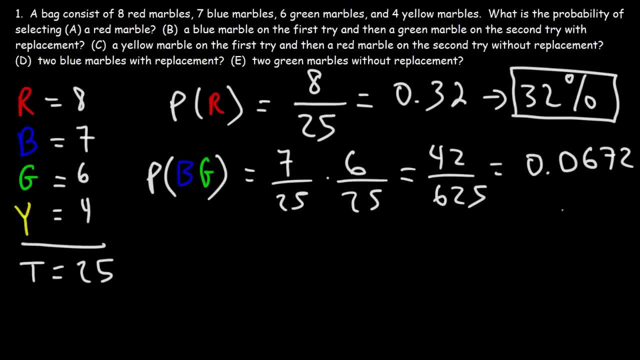 two. So if we multiply that by a hundred, that corresponds to a six point seven, two percent chance of getting a blue marble on the first try and then a green marble on the second try. Now let's move on to part c. What is the probability of selecting a yellow marble on the first? 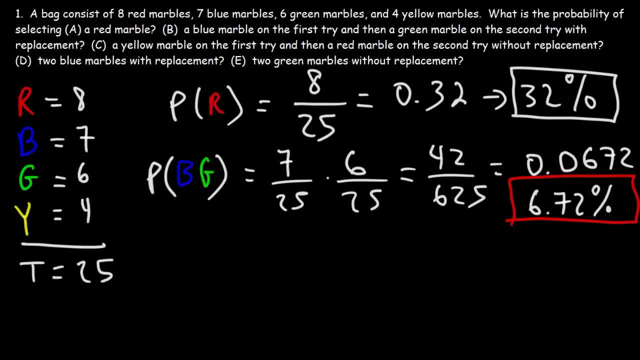 try and then a red marble on the second try without replacement. So what do you think the answer is going to be for that one? So let's start with the first event. What is the probability of selecting a yellow marble? There's four yellow marbles out of a total of twenty five, So it's four out of twenty. 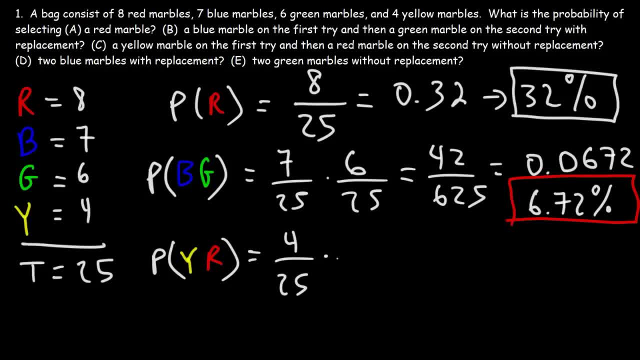 five. Now what do you think the expression without replacement means? This means that once we take out that yellow marble, we are not going to put it back into the bag. So we no longer have twenty five marbles in the bag, But we now have twenty four marbles. 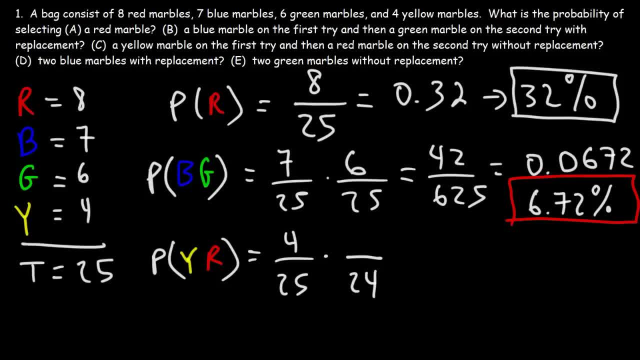 Now we still have eight red marbles. So to select a red marble on the second try it's going to be eight over twenty four, as opposed to eight over twenty five. So let's do the math. Twenty four. I'm going to write that as eight times three and eight. 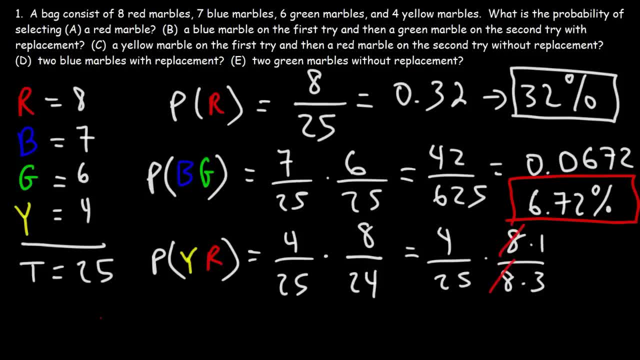 I'm going to leave it as eight times three. I'm going to leave that as eight times three times 1.. So we could cancel. the 8's 25 times 3 is 75. So the probability will be 4 over. 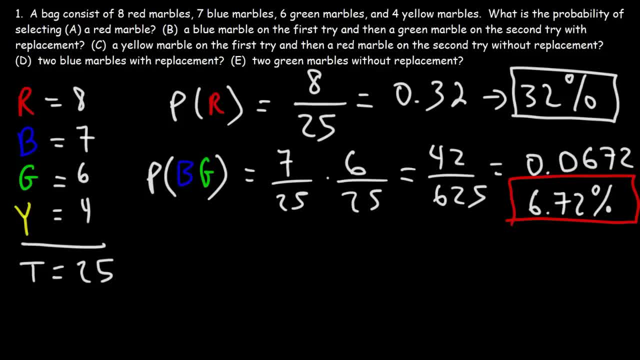 try and then a red marble on the second try without replacement. So what do you think the answer is going to be for that one? So let's start with the first event. What is the probability of selecting a yellow marble? There's four yellow marbles out of a total of twenty five, So it's four out of twenty. 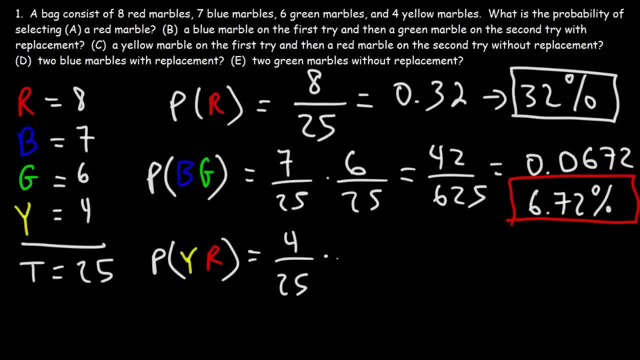 five. Now what do you think the expression without replacement means? This means that once we take out that yellow marble, we are not going to put it back into the bag. So we no longer have twenty five marbles in the bag, but we now have twenty four marbles. 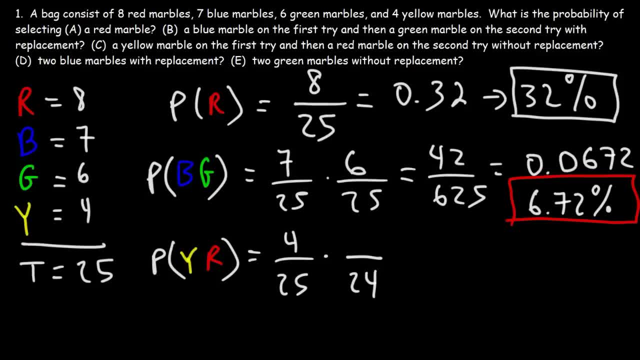 Now we still have eight red marbles. so to select a red marble on the second try it's going to be eight over twenty four, as opposed to eight over twenty five. So let's do the math. Twenty four. I'm going to write that as eight times three And eight. I'm going to leave. 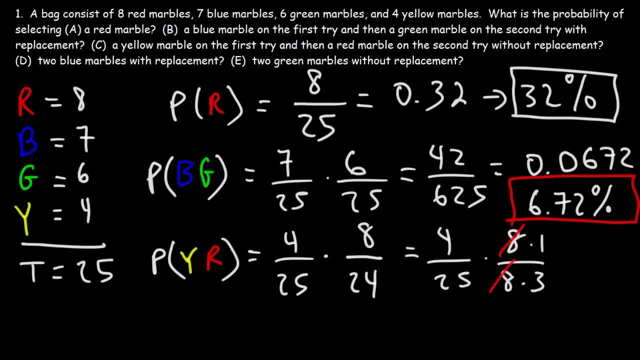 times 1.. So we could cancel the 8's. 25 times 3 is 75.. So the probability will be 4 over 75.. 4 divided by 75 is .053, with the 3 repeated, So this is approximately a 5.3% chance of. 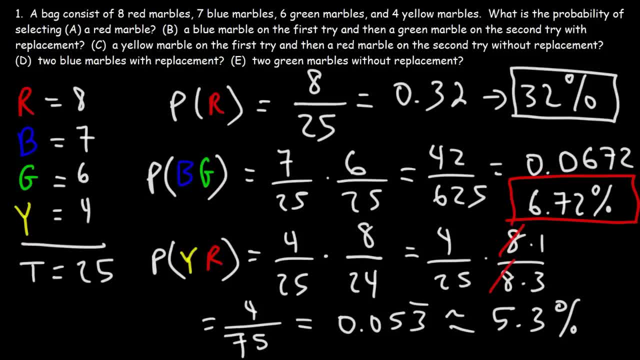 occurring, That's for this particular event. Now let's talk about what we have here: Which situation represents an independent event and which one would you say are dependent events? So part B, there's two events: Getting a blue marble and then a green marble Would 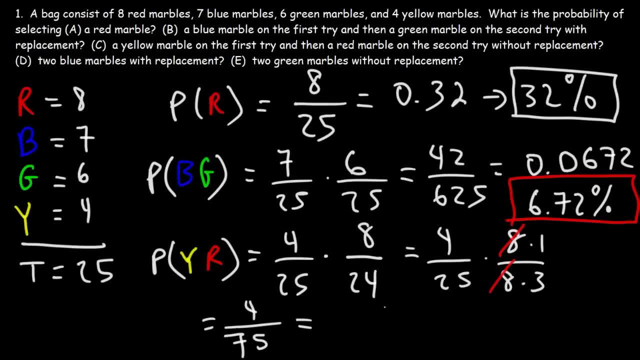 75.. 4 divided by 75 is .053, with the 3 repeated. So this is approximately a 5.3% chance of occurring. That's for this particular event. Now let's talk about what we have here. Which situation represents an independent event and which one, would you say, are dependent? 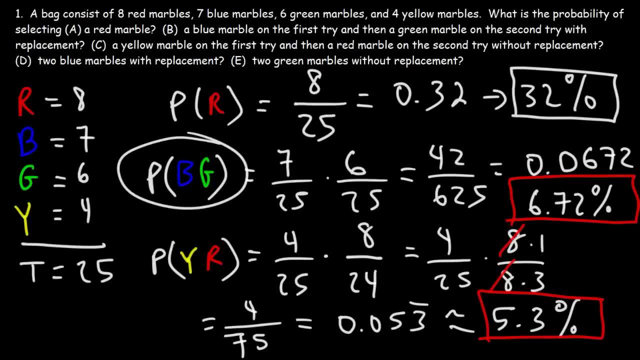 events. So part B, there's two events: Getting a blue marble and then a green marble, Would you say. the second event depends on the first event. What is the probability of getting a green marble? Just of getting a green marble? It's going to be the 6 green marbles out of the total. 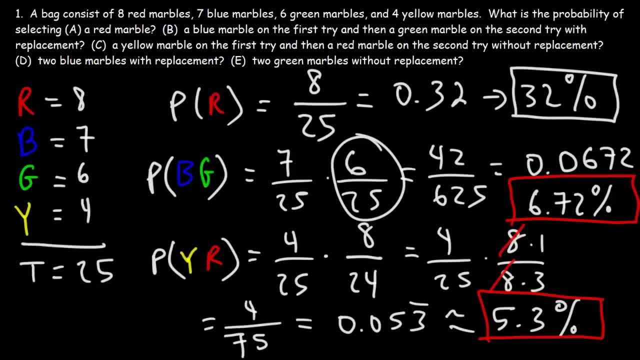 of 25.. And notice that is what we see in the second event. The probability hasn't changed. So getting a blue marble on the first try had no effect on the probability of getting a green marble on the second try. So part B represented a situation with independent 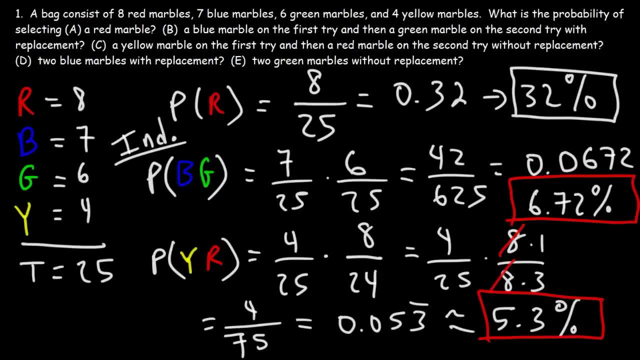 events. Now what about part C? The probability of getting a red marble is 8 over 25.. Did that probability change? Does the second event depend on the first event? Yes, it does, Because without replacement, the number of marbles 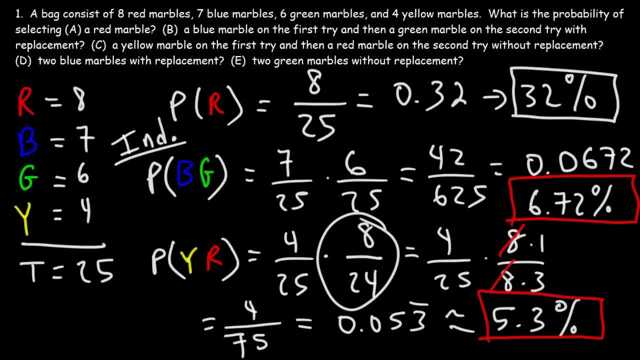 in the bag changes, And so, after you take out that first marble, you no longer have 25 marbles, You now have 24.. And so since the number of marbles in the bag changes, the probability of the second event will change. 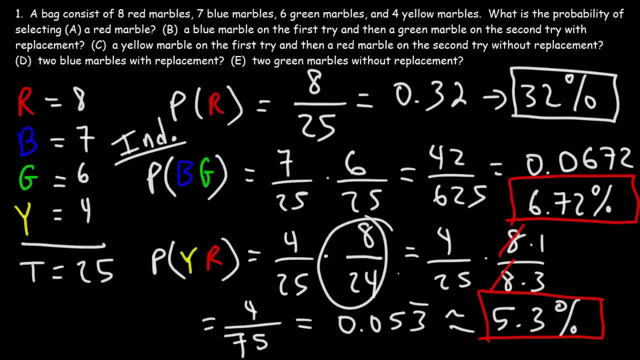 What is the probability of getting a red marble? The probability of getting a red marble is 8 over 25.. Did that probability change? Does it change? Yes, it does. Now we're left with just the red marbles in the bag. 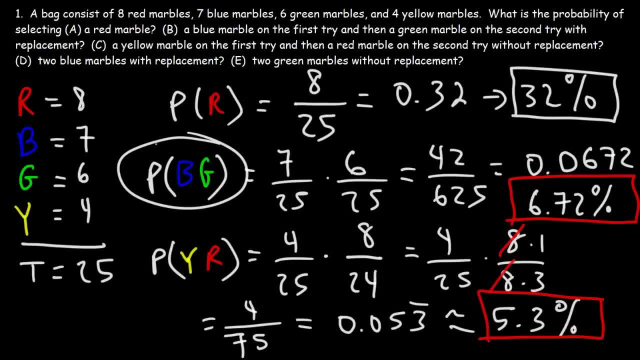 you say the second event depends on the first event. What is the probability of getting a green marble, Just of getting a green marble? It's going to be the 6 green marbles out of the total of 25.. And notice, that is what we see in the second event. The probability hasn't changed. 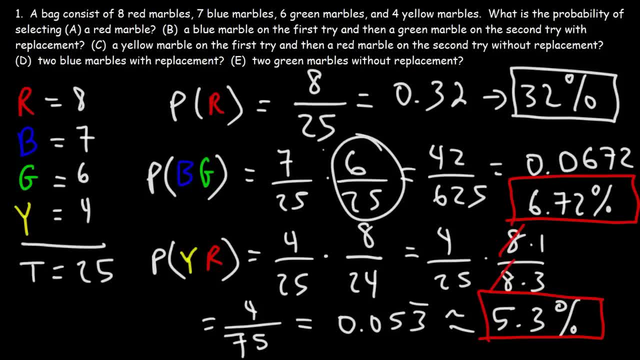 So getting a blue marble on the first try had no effect on the probability of getting a green marble on the second try. So part B represented a situation with independent events. Now what about part C? The probability of getting a red marble is 8 over 25.. Did that probability change? Does 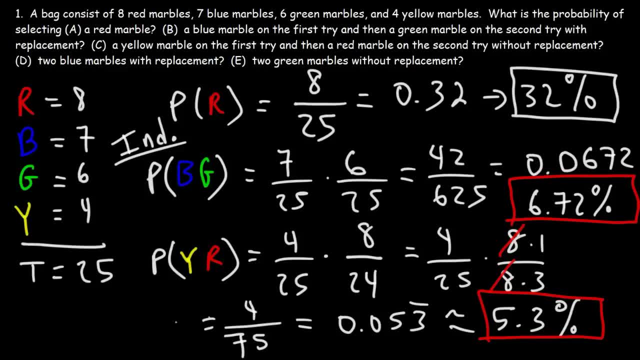 the second event depend on the first event? Yes, it does, Because without replacement, the number of marbles in the bag changes. And so, after you take out that first marble, you no longer have 25 marbles, You now have 24.. And so, since the number of marbles in 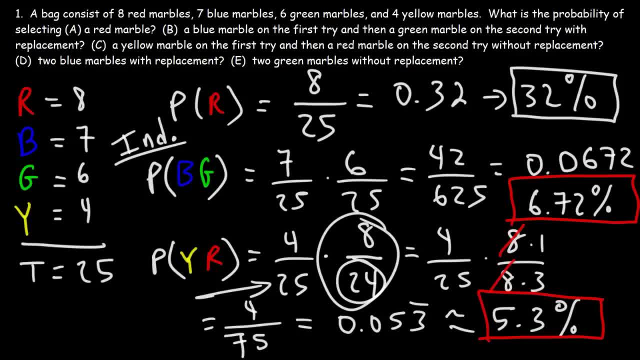 the bag changes, The probability of the second event will change. As you can see, the second event is 8 out of 24, compared to what it would be, which would be 8 out of 25, if we didn't select the yellow marble on the first try, without replacement. 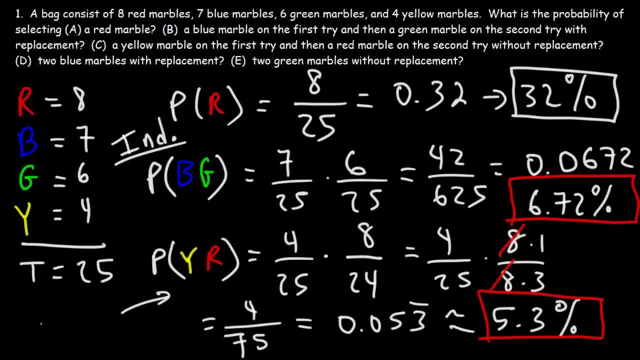 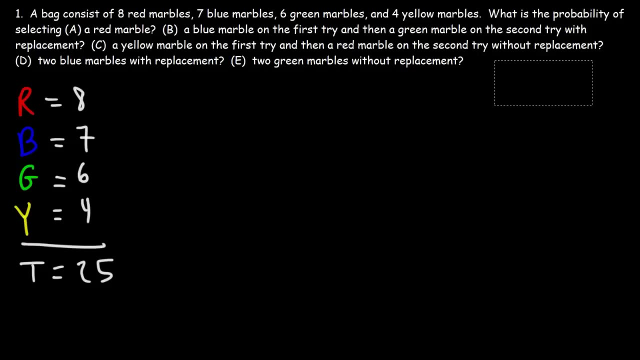 So anytime you have a situation where it's without replacement, you're dealing with dependent events. When it's with replacement, you're dealing with independent events. So keep that in mind. Now let's move on to part D. What is the probability of selecting two blue marbles with replacements? 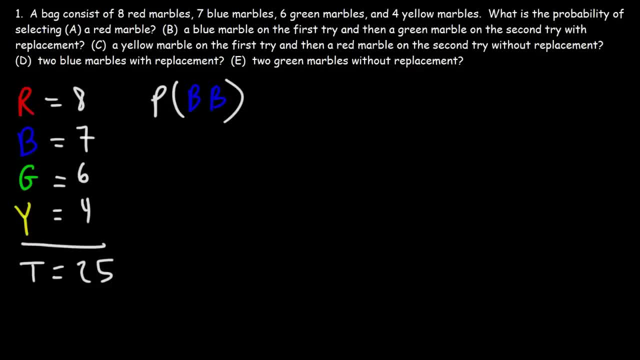 So is this going to be dependent events or independent events? Since it's with replacement, we're dealing with With independent events, So the probability of getting the first blue marble is 7 out of 25.. Now we're going to put that blue marble back in, So we're still going to have a total. 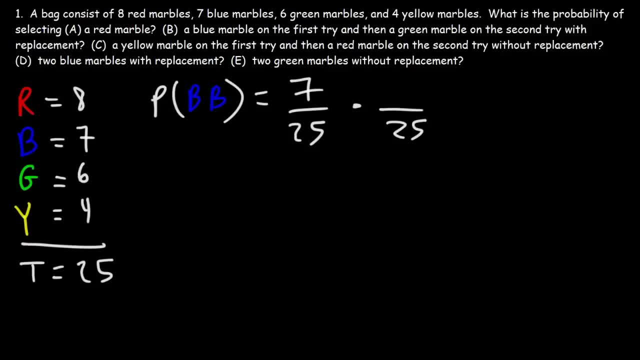 of 25 marbles And it's still going to be 7 blue marbles. So on the second try, the probability will not change. 7 times 7 is 49.. 25 times 25 is 625.. So this is equal to. If you are trying to get an 8 out of 24 marble, the probability of getting a red marble in the bag is 8 out of 25.. Now you can see the second event is 8 out of 24 compared to what it would be, which would 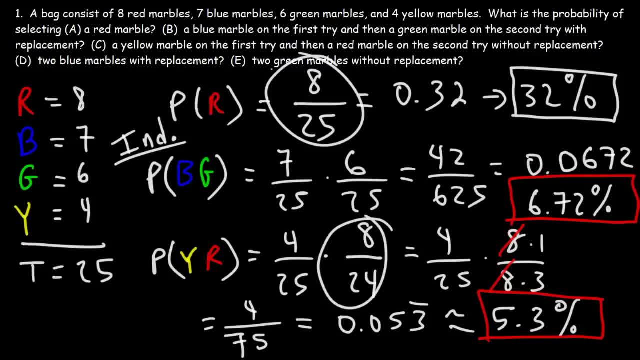 be 8 out of 25, if we didn't select the yellow marble on the first try without replacement. So any time you have a situation where it's without replacement, you're dealing with dependent events. When it's with replacement, you're dealing with independent events. So keep that. 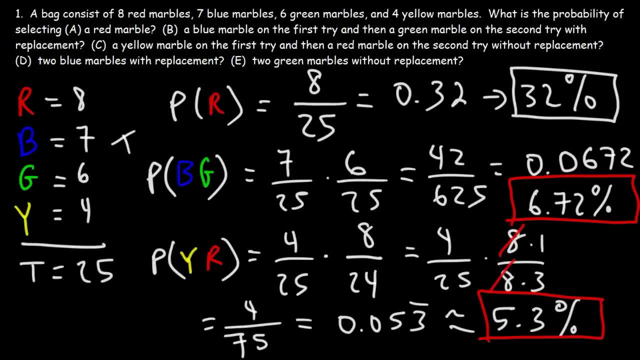 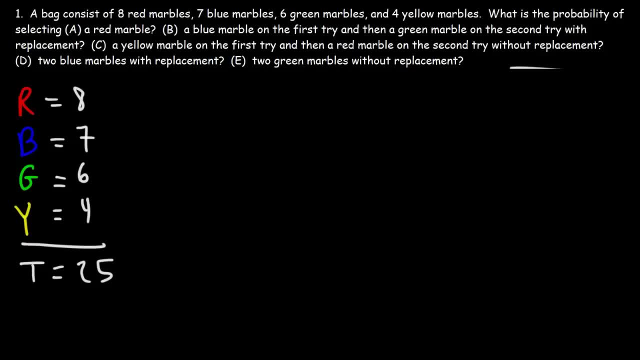 in mind: Part D, Part B, Part C, Part D, Part C, Part B. What is the probability of selecting two blue marbles with replacements? So is this going to be dependent events or independent events? Since it's with replacement, we're dealing with independent events. 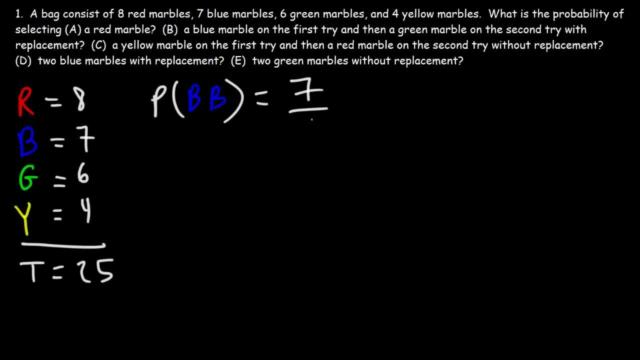 So the probability of getting the first blue marble is 7 out of 25.. Now we're going to put that blue marble back in, So we're still going to have a total of 25 marbles and it's still going to be 7 blue. 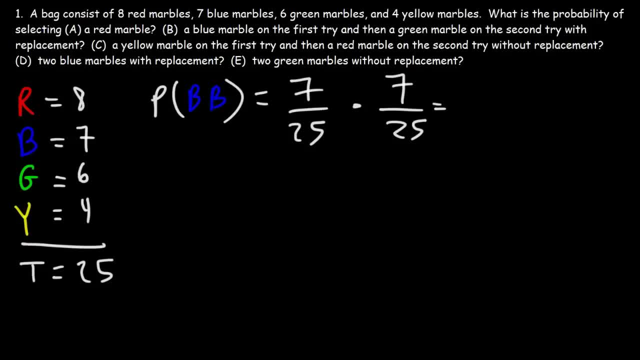 marbles. so on the second try, the probability will not change. Seven times seven is 49,. 25 times 25 is 625.. So this is equal to 0.0784.. Okay, So there's a 7.84% chance of selecting two blue marbles with replacement. 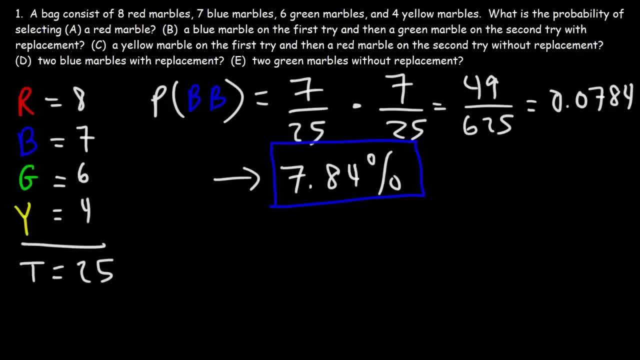 Now part E: what is the probability of selecting two green marbles without replacement? So now we're dealing with dependent events. So we have six green marbles out of a total of 25.. Now, once we take out one green marble, We now only have 24 marbles in the back. 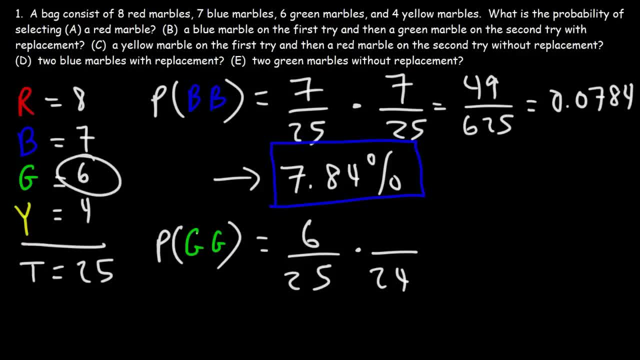 Now we don't have six green marbles anymore, Because we took out one. we now have five green marbles, And so this is the situation that we now have. Let's write 25 as five times five, And let's write 24 as six times four. 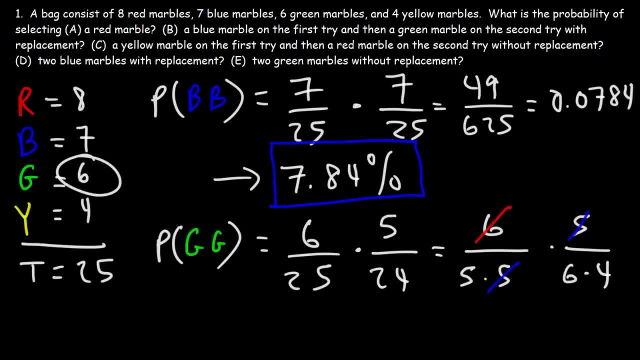 So we could cancel a five and we can cancel a six. So since there are no more numbers on top, We can cancel a six. We're just going to put a one. On the bottom. we have five times four, which is 20.. 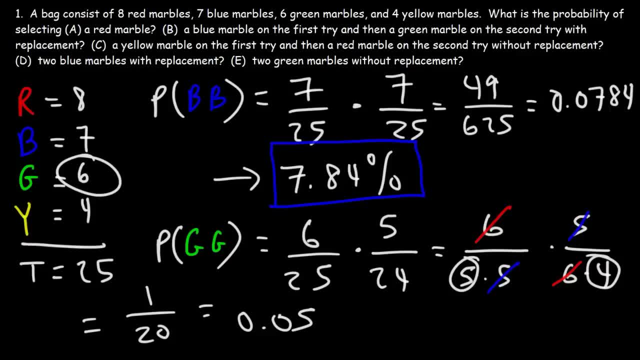 One divided by 20 is 0.05.. So if we multiply that by 100. This tells us that there's a 5% chance of selecting two green marbles without replacement.